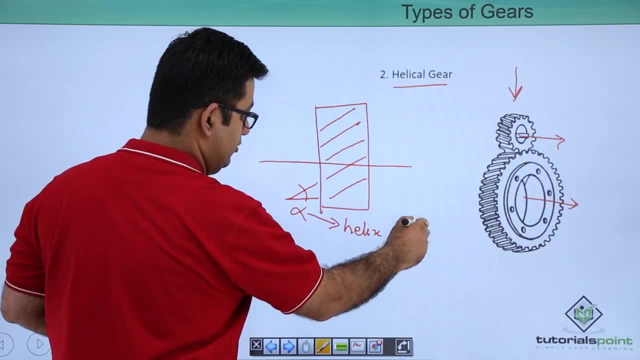 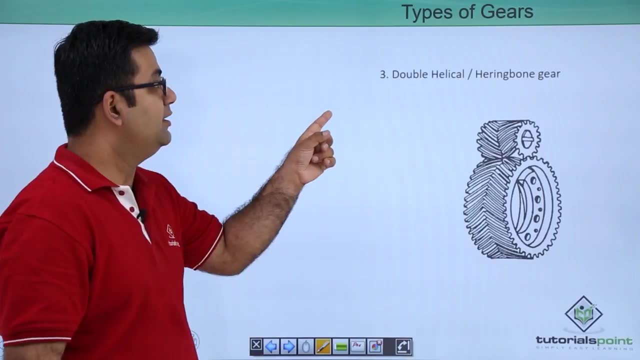 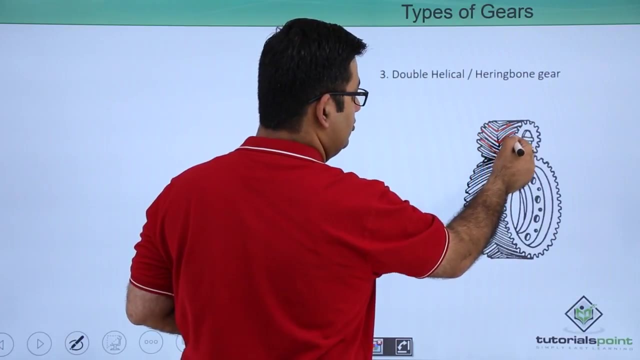 it is known as the helix angle. alright, so this is a single helical gear. this is a double helical gear because you can see that in this there are two angles at which the teeth is inclined to. so, again, the shaft axis are parallel, like this, like: 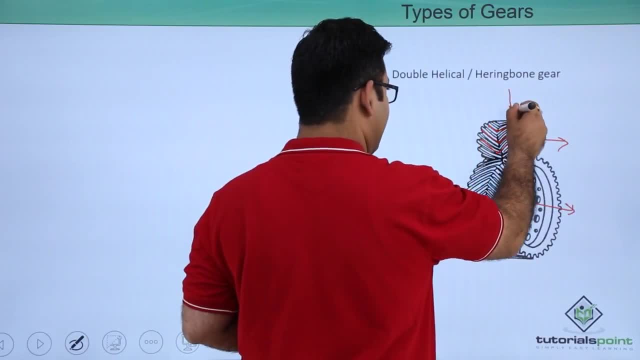 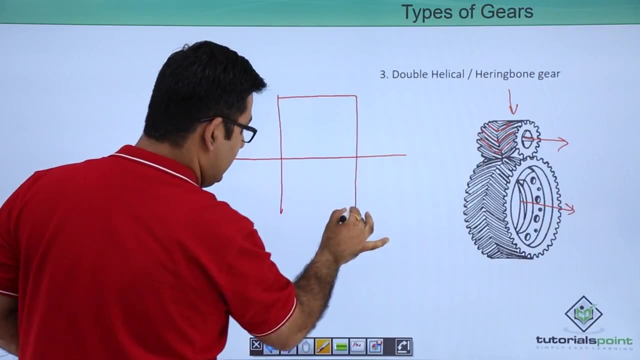 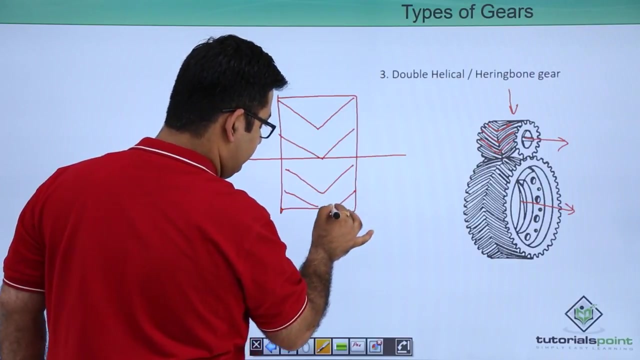 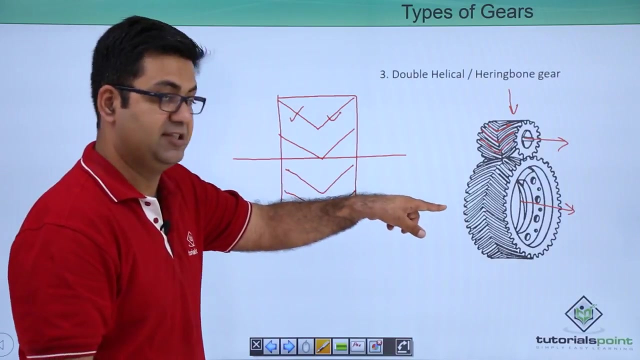 this, but when you look at this kind of a gear from the top and you see the plan of it, okay, so this is the shaft axis, this is how the gear looks like and it will be having teeth like this. So you can see that this is one helix, this is the second helix, so you have double helix. 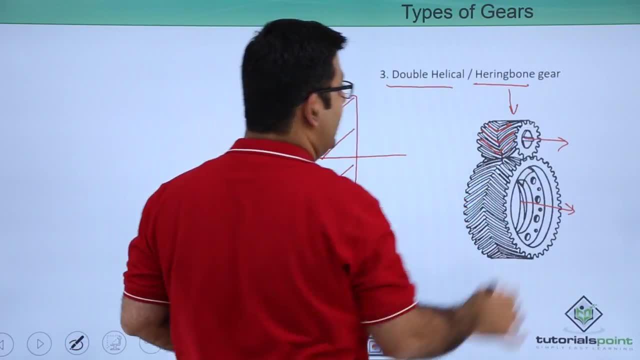 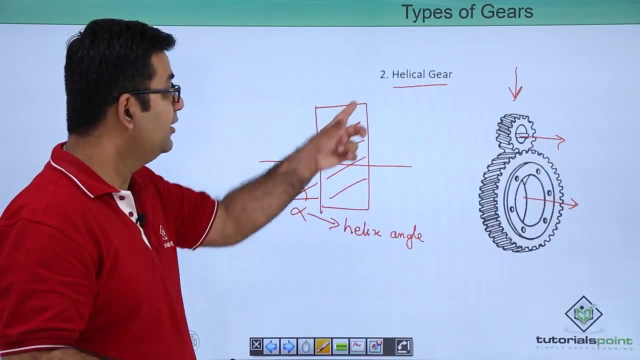 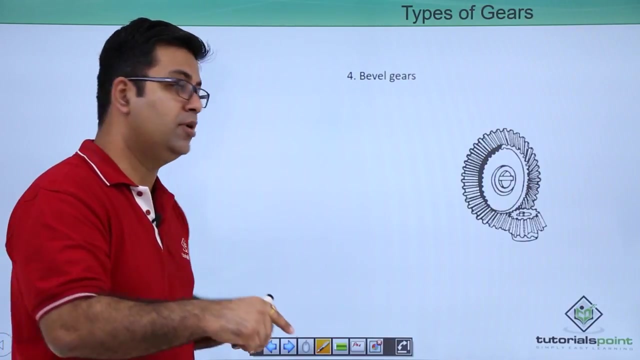 in this. that is why it is called a double helical or a herringbone gear. so in a herringbone gear the power transmitting capacity is higher as compared to the single helical gear. okay, so from spur helical herringbone we come to the bevel gears. now, what are bevel gears? 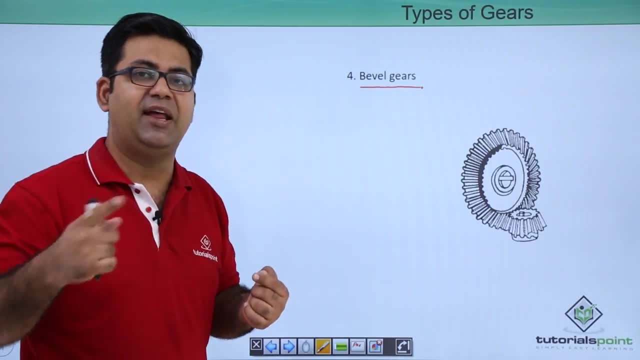 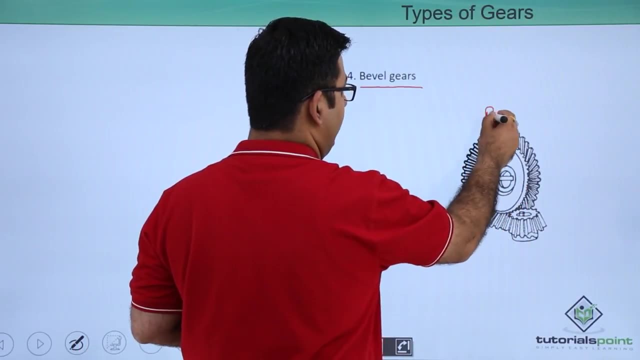 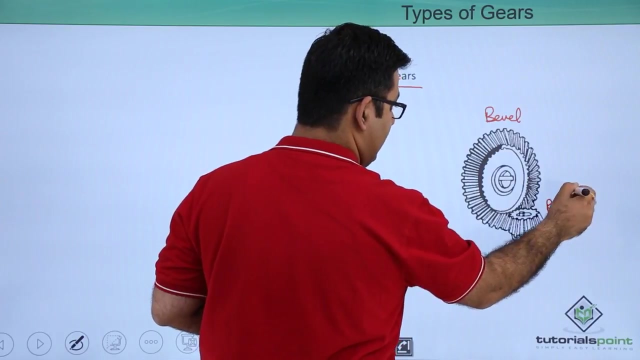 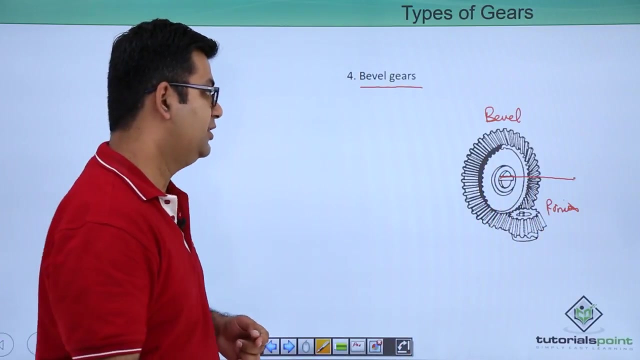 bevel gears are those gears in which the shaft axis are intersecting at ninety degrees to each other. okay, so if you look at this bigger gear, which is known as the bevel, okay, the smaller gear is the pinion. it is the pinion. okay, so the axis of this bevel is, let us say, 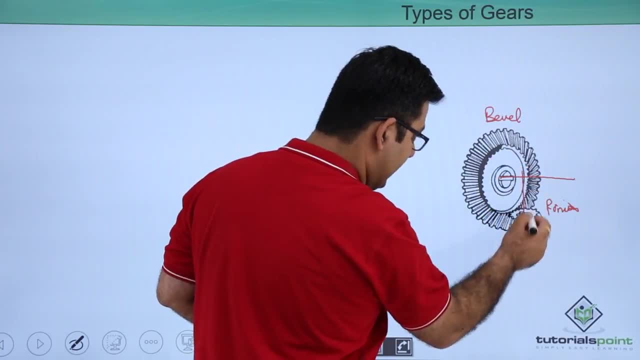 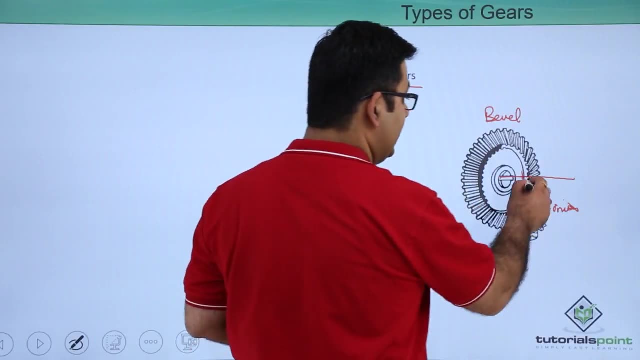 like this, and the axis of this pinion would be vertical like this. So you can very clearly see that the axis of these two gears are intersecting and they are intersecting at ninety degrees to each other. okay, so in a nutshell, I can say that. 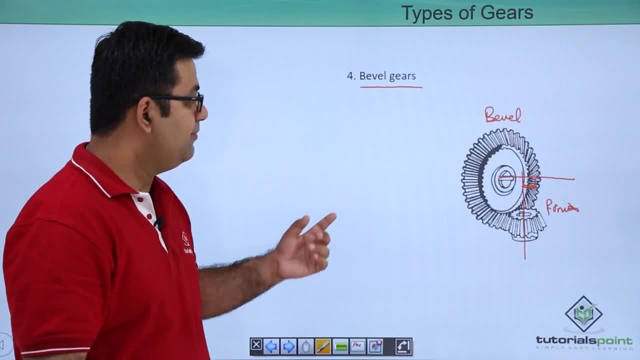 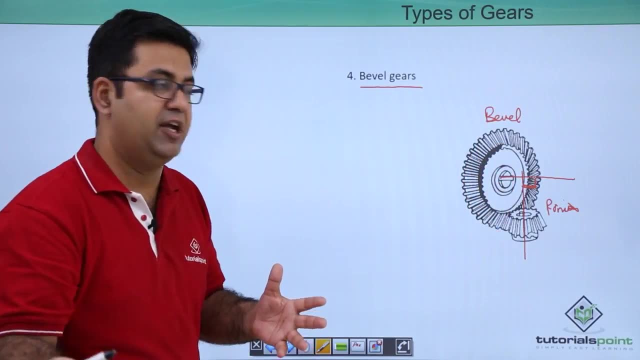 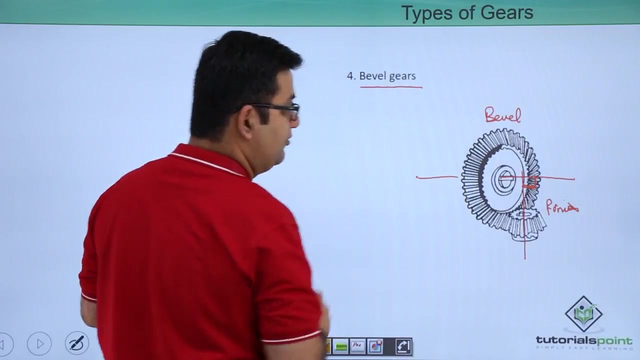 a bevel gear arrangement is used where the power transmission is at ninety degrees. so the prime mover, let us say this bevel is the you can say driven and this is the driver, or whatever the case is, This axis is for the driver, Okay, 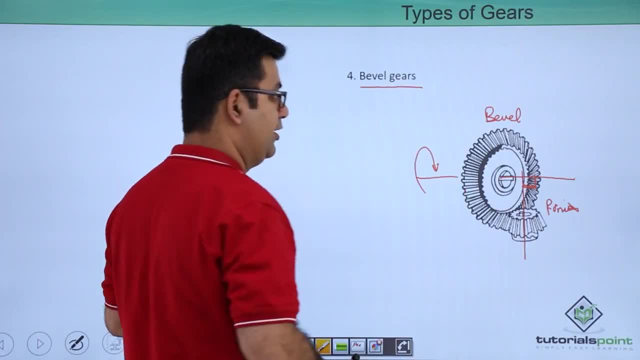 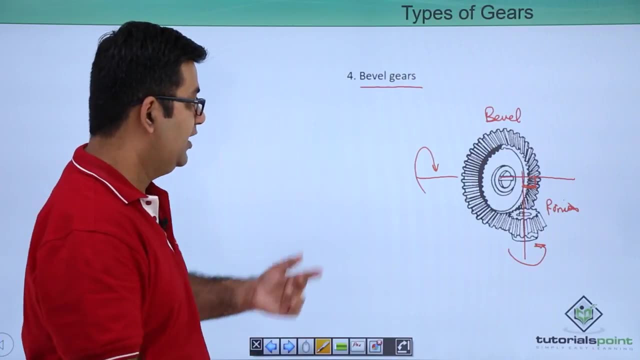 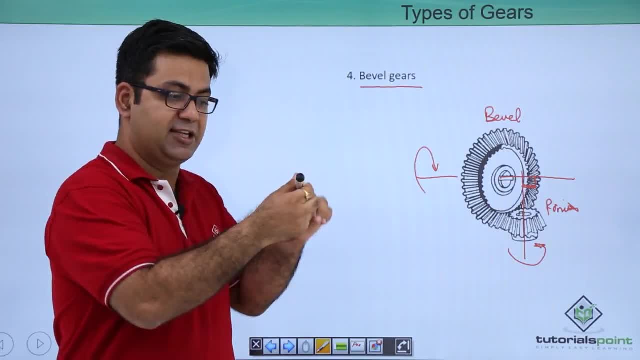 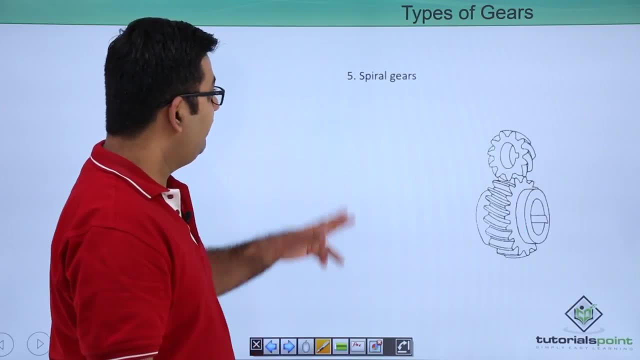 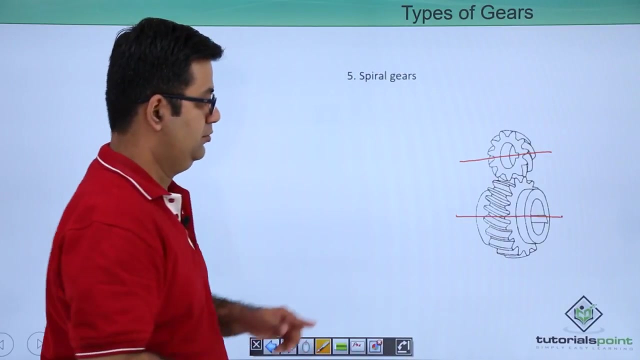 in which the rotation is like this. the pinion axis would be like this: at ninety degrees, with rotation like this: okay, after bevel, we come to the spiral gears. so now, in spiral gears, you have. Okay, So you can see that the shafts are not parallel, and you can see the shafts are not parallel. 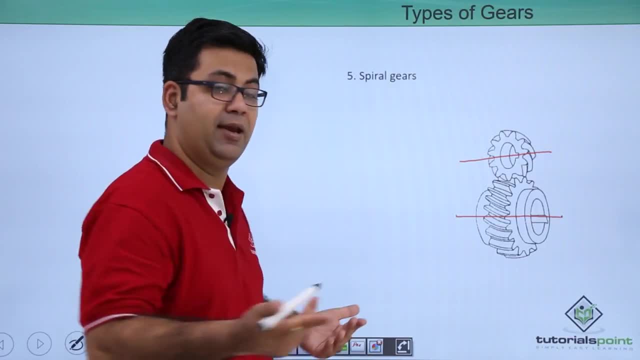 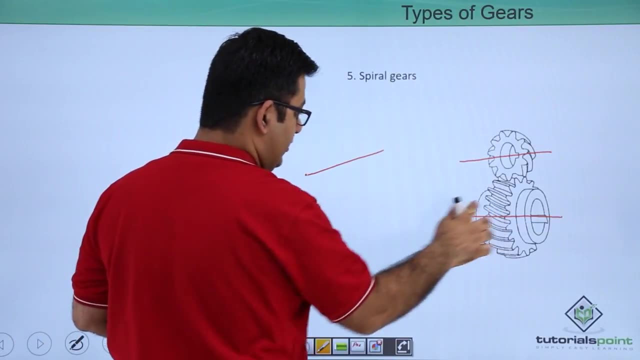 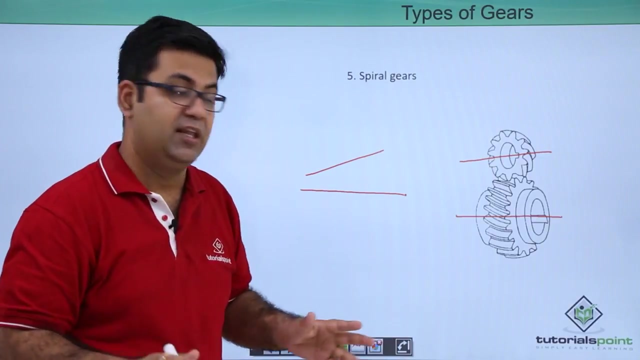 in this kind of a shaft axis. so in this the shafts are neither parallel, not they intersect. so if you look at it from the top, this is, let us say, going over here and this one is, let us say, going over here. So from top they might seem that they would intersect somewhere over here. but no, they. 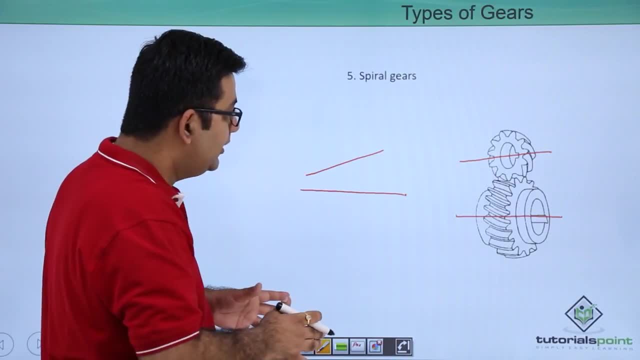 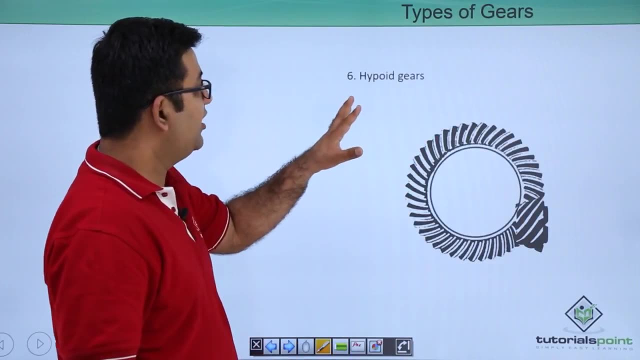 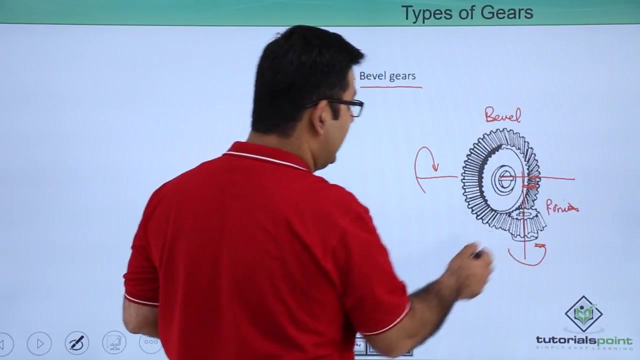 are not lying in the same plane, They don't intersect. okay, they are not parallel, so they are called spiral gears. Okay, Okay, Okay, Okay, Okay. The next kind of gear is the hypoid gear. So if you come back to the bevel gears, in bevel gears you can see that your axes are intersecting. 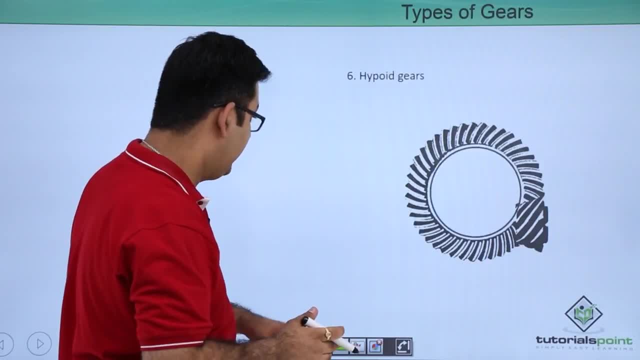 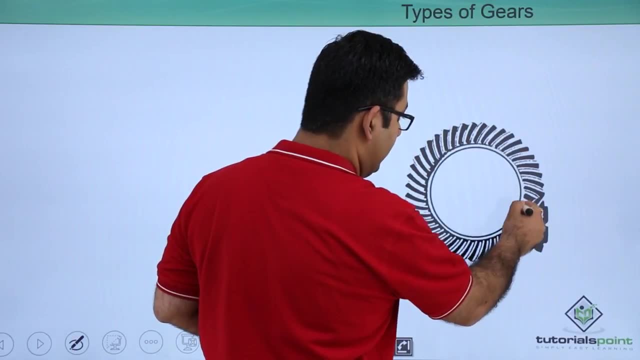 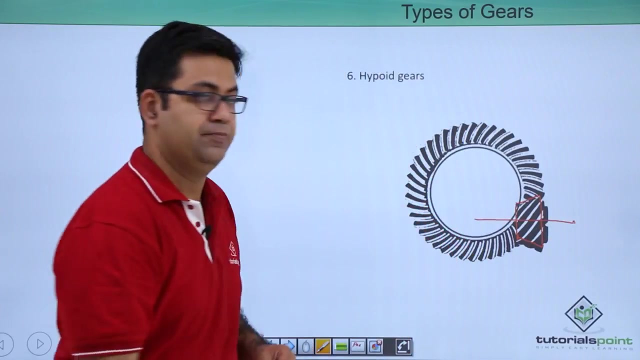 There is intersection of the two shaft axes, but in hypoid gears there is no intersection. So if you look at the axis of this pinion over here, this is the pinion. The axis of this pinion is this, So it is rotating in this plane. 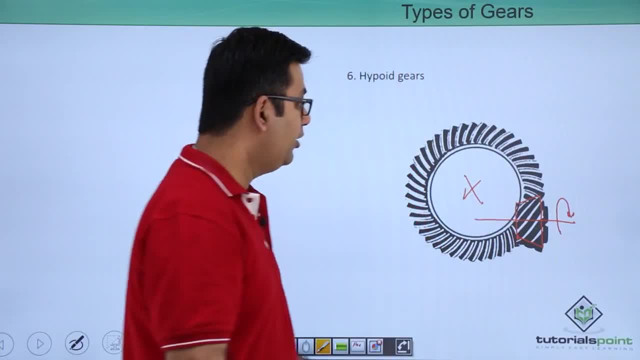 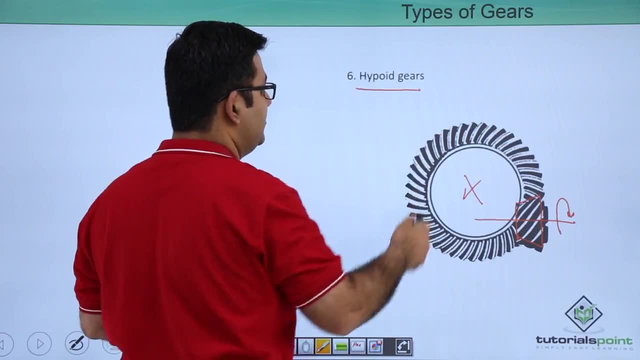 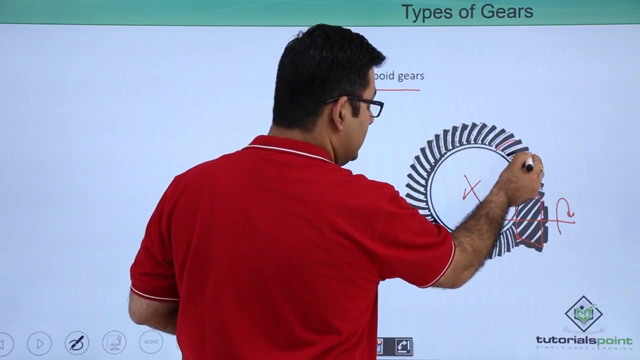 The axis of this gear is perpendicular to the plane of the screen, So neither they will intersect nor they are parallel. So hypoid gears are special kind of bevel gears with inclined teeth on the bigger gear like this You can see If you go back to the bevel gear. 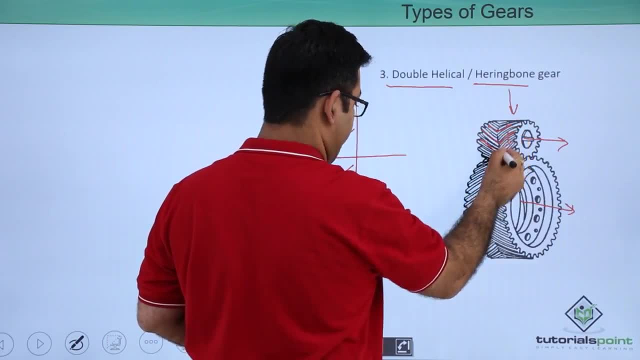 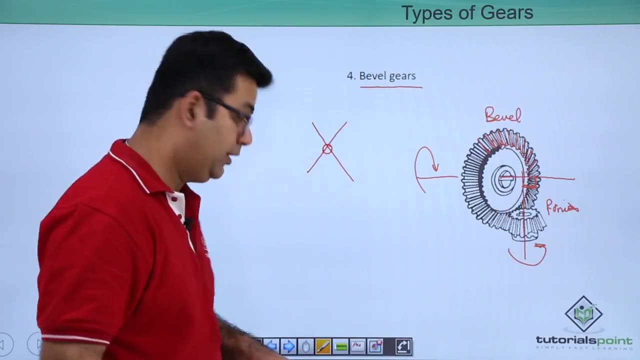 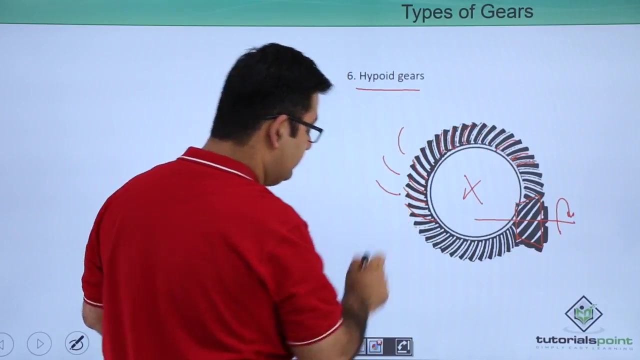 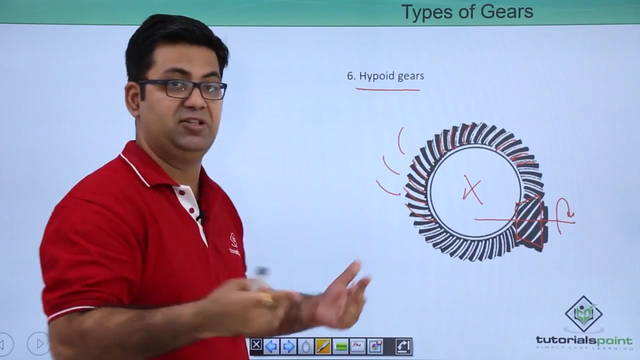 they turn like this: The teeth are straight. The teeth are straight, But in the hypoid gears the teeth are inclined like this And in bevel gears there was an intersection of the axes at 90 degrees, but in this there is no intersection. 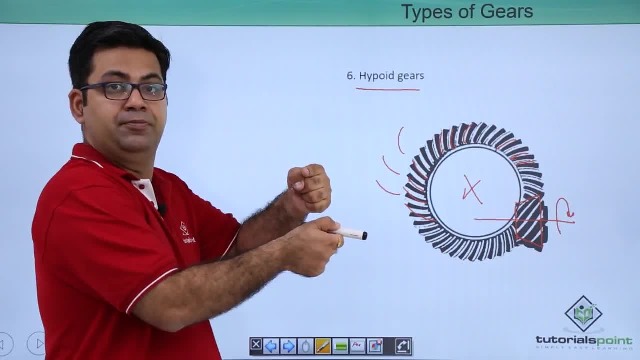 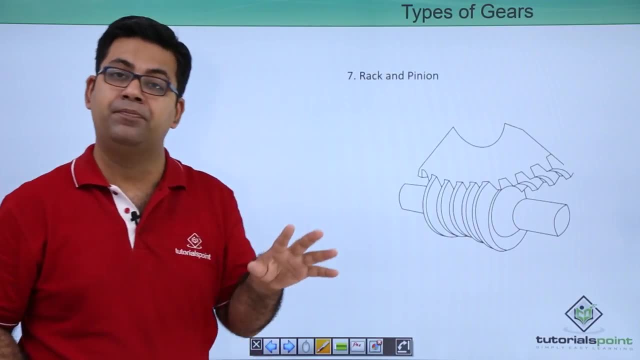 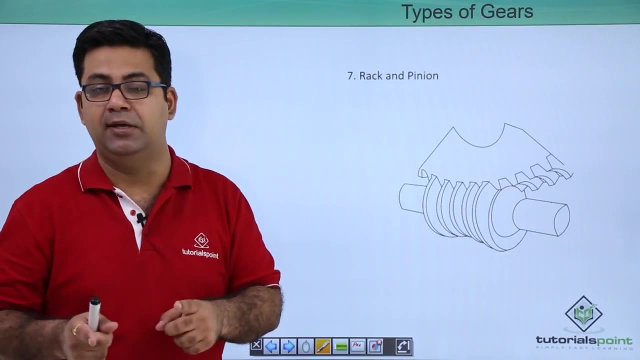 So one is like this and the other one is like this. So there is no intersection, Neither they are parallel. The last one is the rack and pinion. Now the bevel and the hypoid gears were used when there is a change in the direction to which the power has to be supplied.